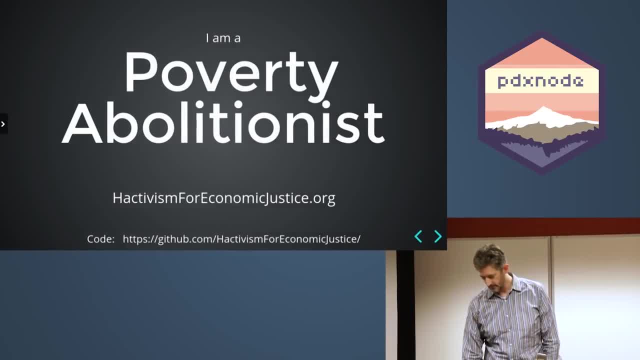 for this on the GitHub there And if you're into it. So what am I doing? I am a web worker. I'm a poverty abolitionist. The world used to be flat. We used to buy and sell people. We used to make kids work in factories. I believe it's time we should abolish poverty. 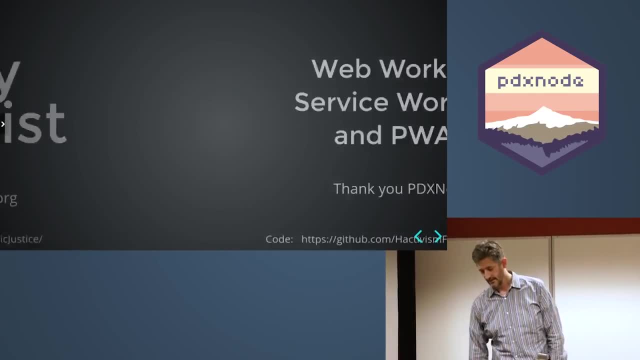 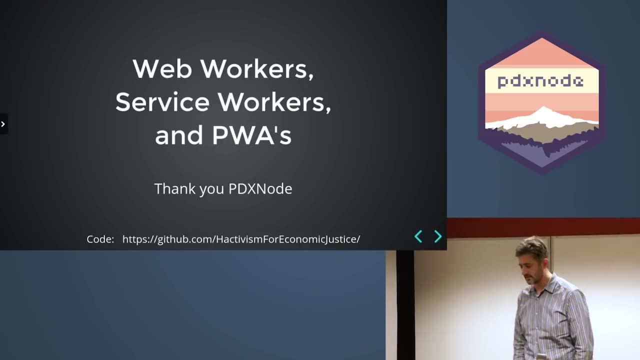 If you're interested in that, come talk to me about it. It's really my jam. If you guys are into it- this hacktivism for economic justice- get in touch with me. through that, I'm looking to find people who are interested in helping out projects around this. But tonight's 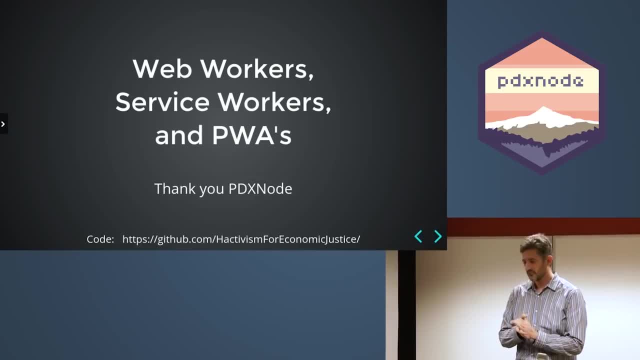 I'm really excited to be here with you guys at PDXNode. We're going to talk about web workers, service workers and PWAs, So I'm sure you all know regular web pages. They're just regular, It's just your HTML. 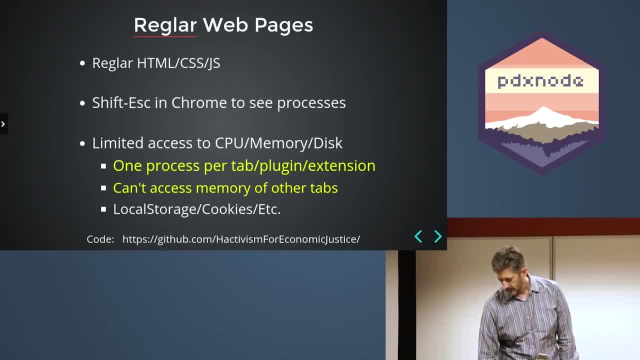 and your CSS. If you do control escape, I can't do it in full screen, But if you do control escape, you can see all the processes that are going on in Chrome. And what's interesting is that the web page- And it's actually really cool about the JavaScript engine- It runs in the event loop And what 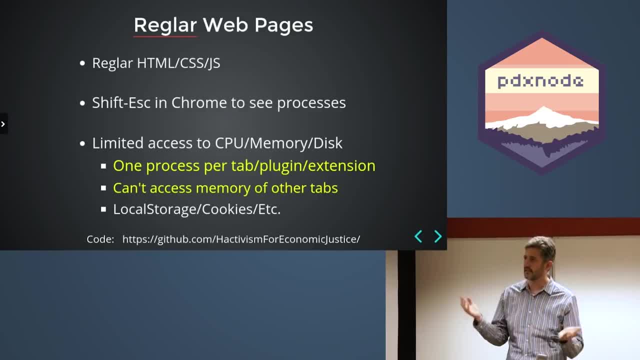 that means is: the code is actually pretty easy to think about, But you also get kind of the simulation of multiple processes and stuff. You can do async stuff, But you really get limited access to CPU disk and memory And you end up with the event loop just being. 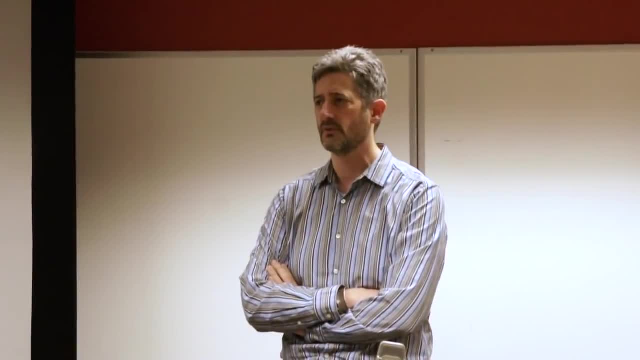 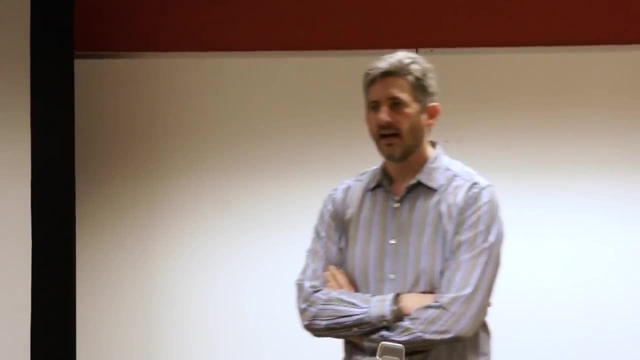 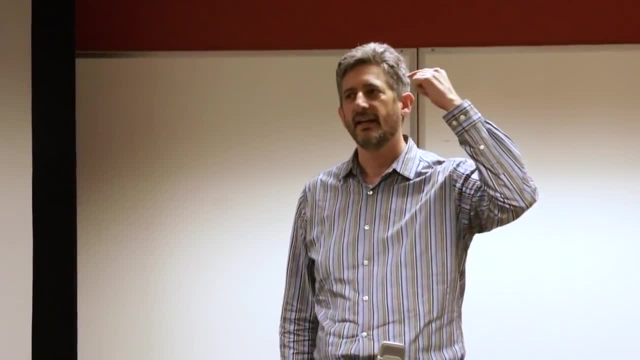 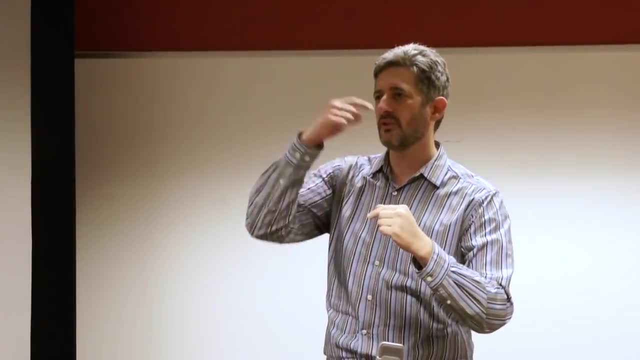 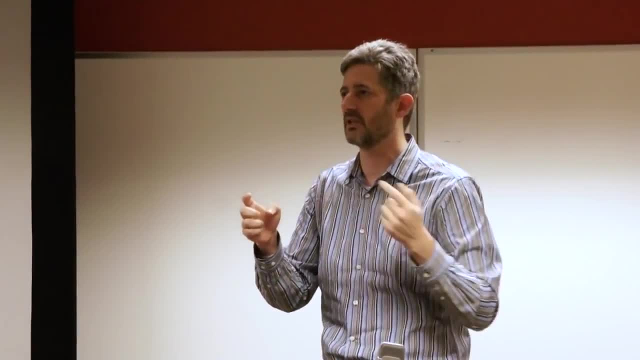 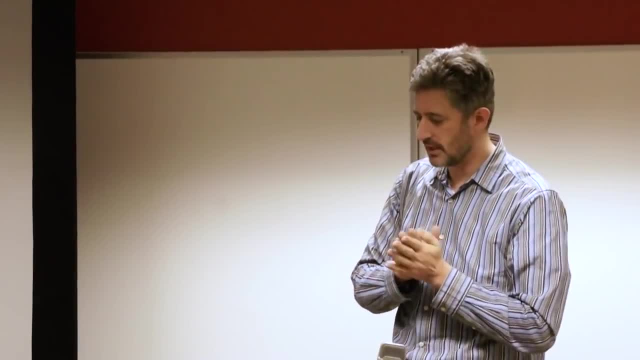 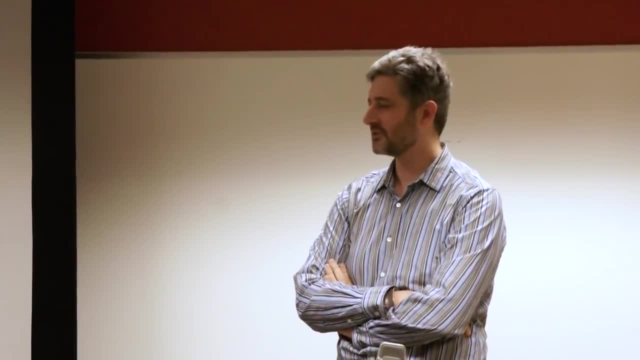 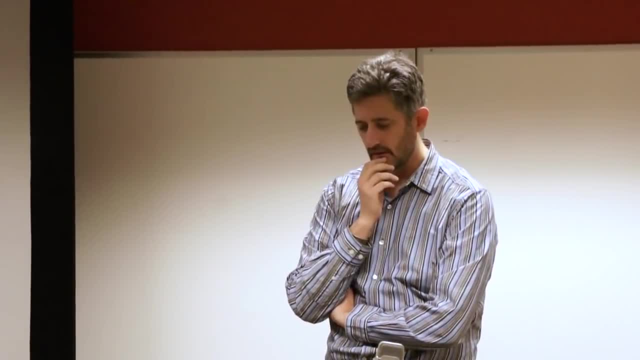 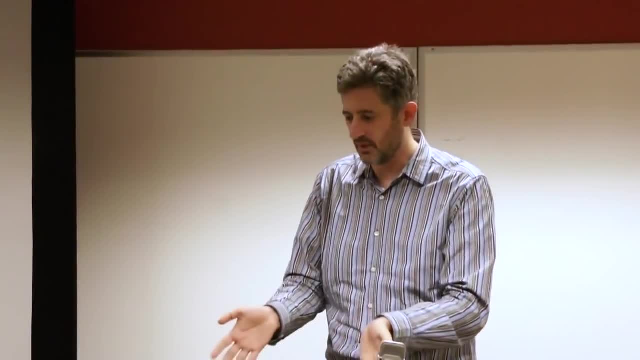 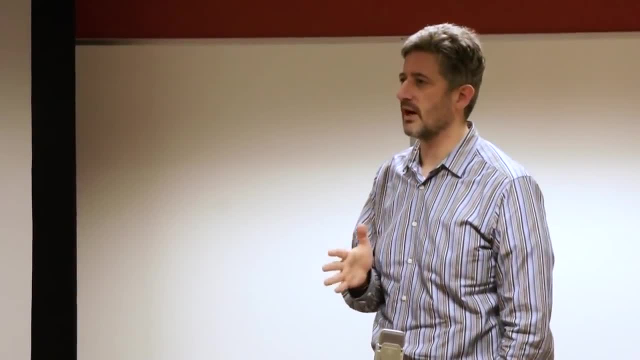 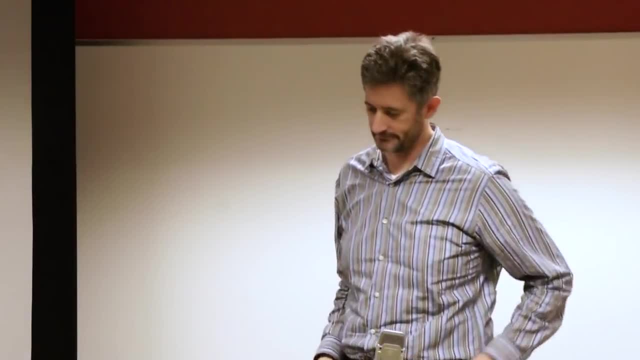 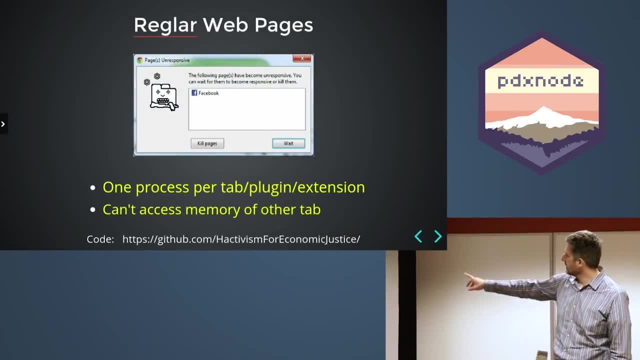 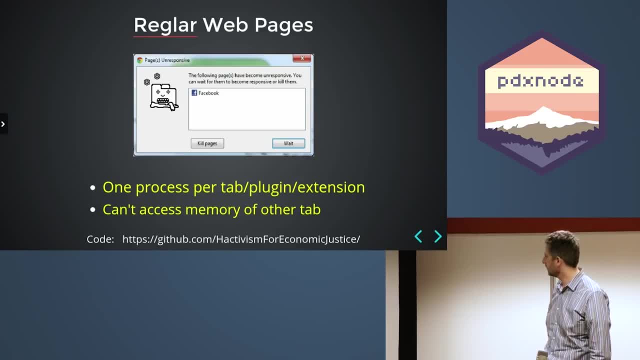 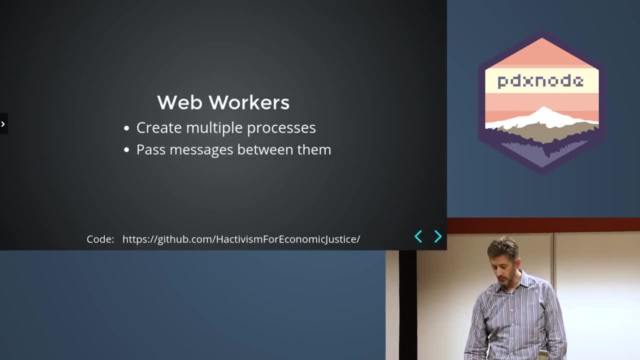 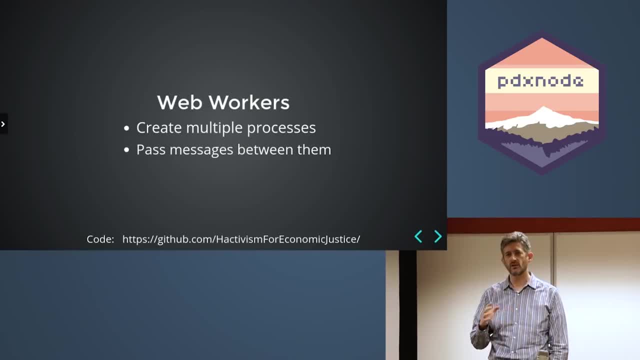 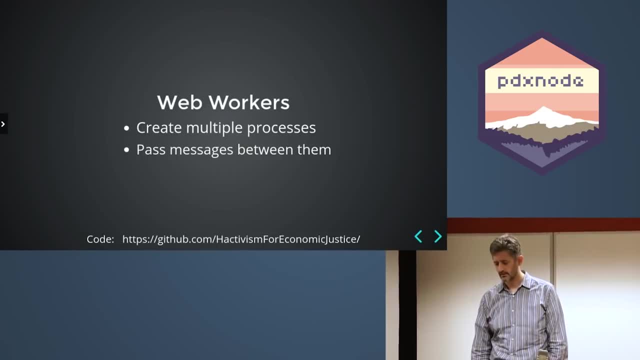 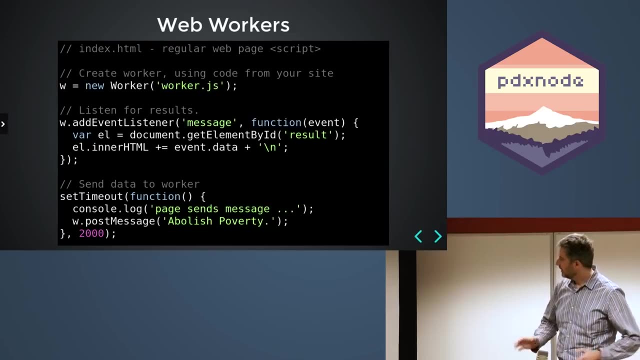 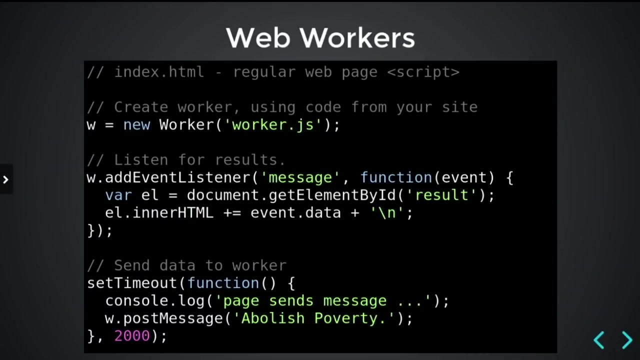 some rules around local storage. you get to get access data that way too. so here's an example of a script tag on a regular web page. you can see, here we're going to create this new worker, and this workerjs is a file to show you here in. 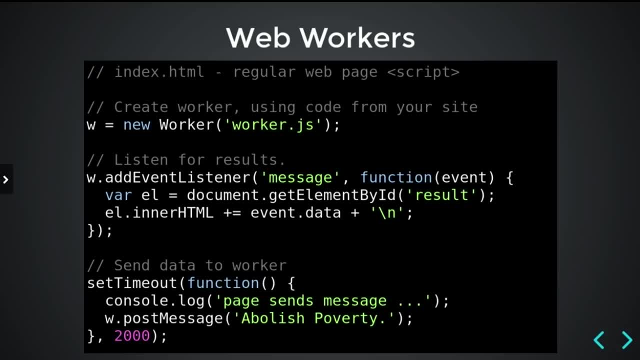 a minute. what we're doing here in this piece of code is we're listening for an event, which is a message event. when that message that happens, we're gonna- we're gonna append some text to this, to this result ID. I'm gonna show you guys this example. if you can just imagine, there's a, an element with the ID result. 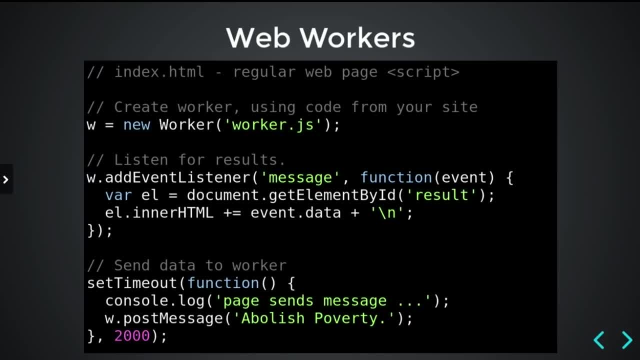 we're gonna actually add to its inner HTML the data from the event, which is which was passed to us in a message. now, here in this, here in this, here in this, this bit here. so this is gonna, this is gonna be what the web worker sends us. 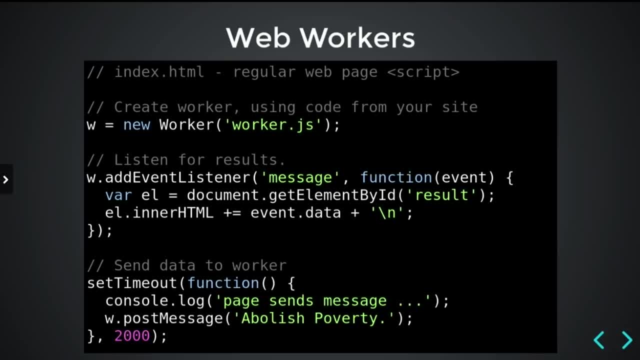 right, so I'm. we are now a web page called indexhtml. when we create web worker, it actually goes up loads of this JS file, and now we're gonna listen for these message events from in this, in this process that's happening on indexhtml- right now this one. what we're gonna do here is we're gonna set a timeout and we. 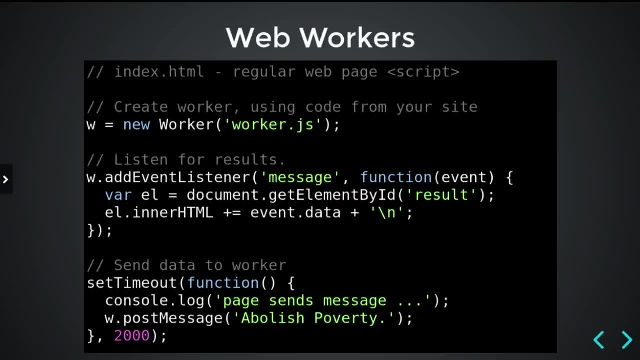 are gonna post a message to the web worker so we can communicate to the web worker through messages and the web worker could communicate to us through messages. right, so this is how we can get like useful stuff in and out of the web worker. the way worker doesn't really have any like data or context available. 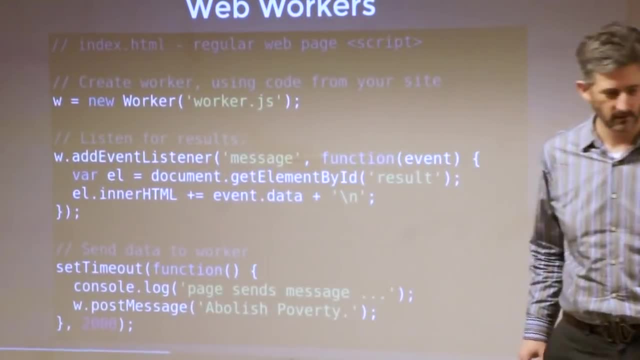 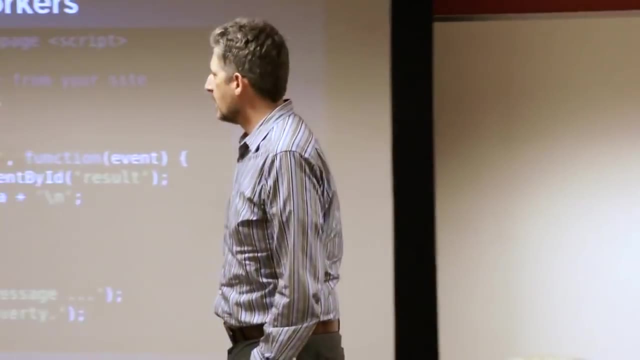 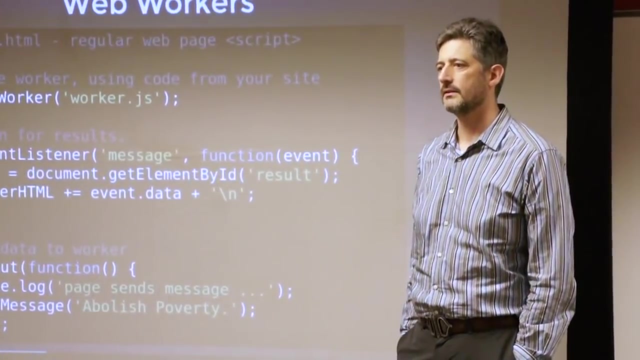 to it, so we really have to send it through through messages. does that? does that make sense? anybody, anybody, have questions about that. yeah, what can you pass it as a message? does that have to be like some simple types like strings, and it's maybe an object with those, but not like a DOM element? 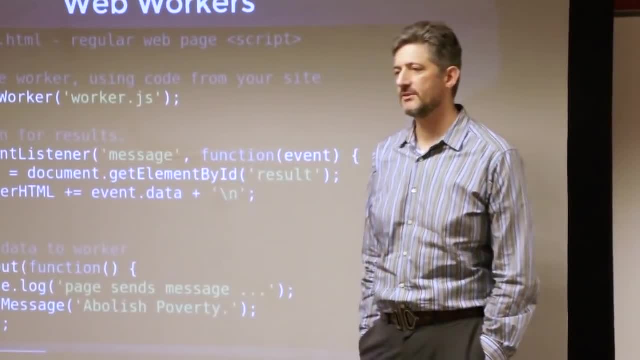 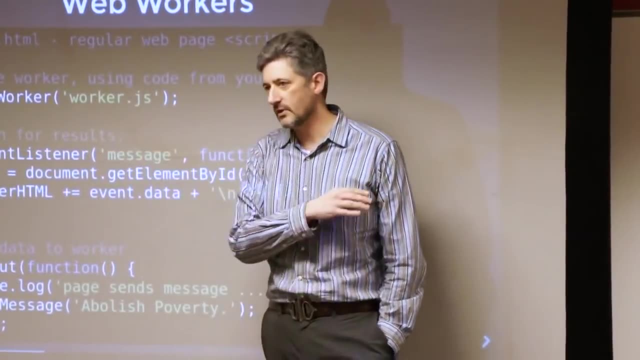 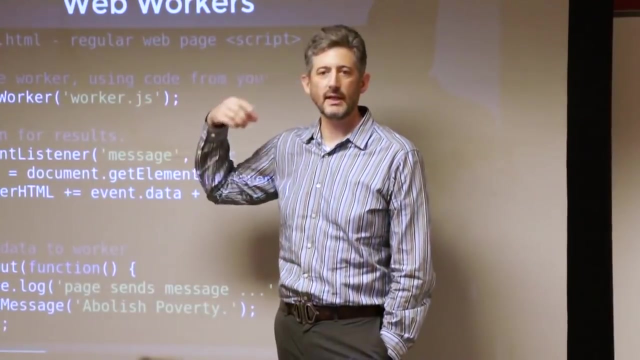 You can pass in a copy of a DOM element. you can pass in a copy of DOM info, but the WebWorker doesn't have any access to the DOM, so you can't use jQuery with it In the WebWorker. you can load in other scripts. so you can load in Lodash and other libraries. 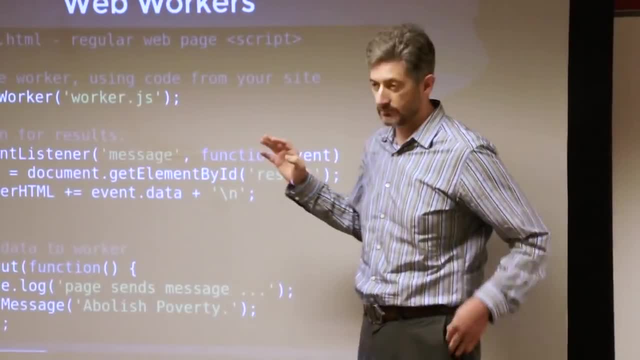 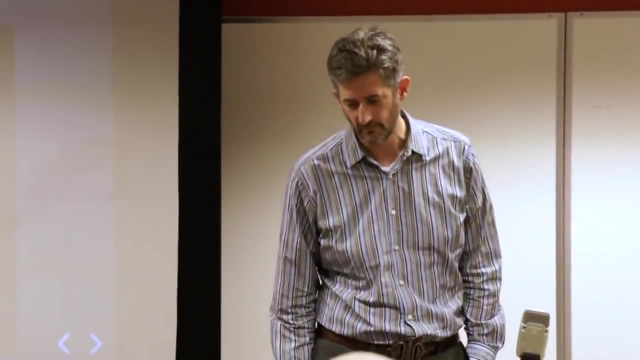 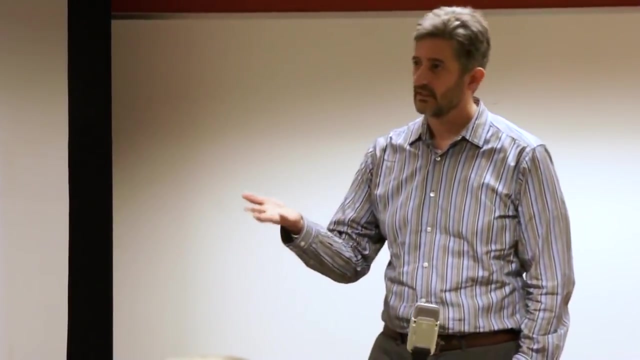 like that, But the data that you pass back and forth has to be a basic data type. I think you can do a JavaScript object, All right, Yes, Or the equivalent of that. whether it actually does that, it just sort of gets a value type. 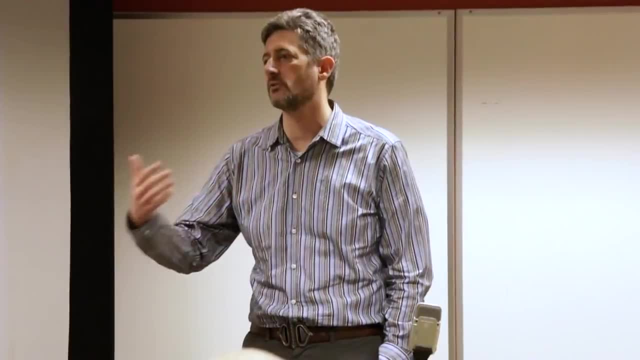 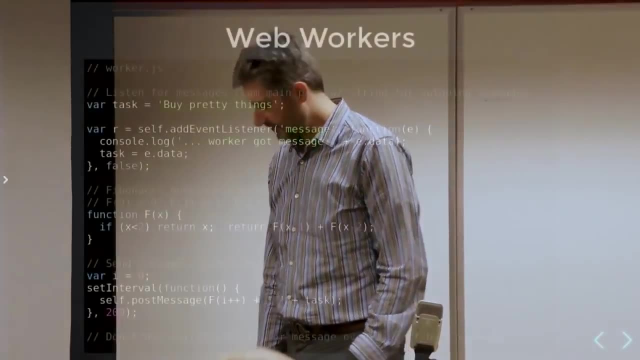 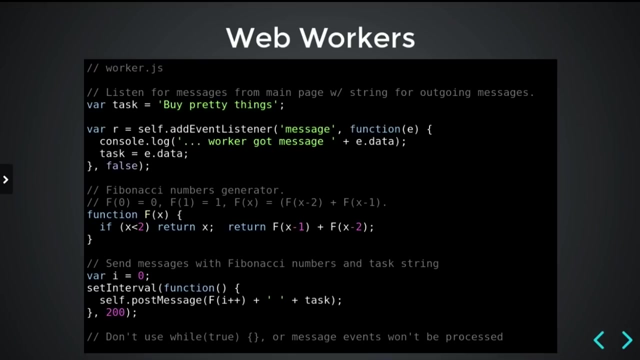 out of it Exactly. yeah, You can't pass a reference, Right, Thank you. Thank you, Okay. So here's our workerjs, Okay, And so we are going to listen for messages from the main page with a string as we wait. 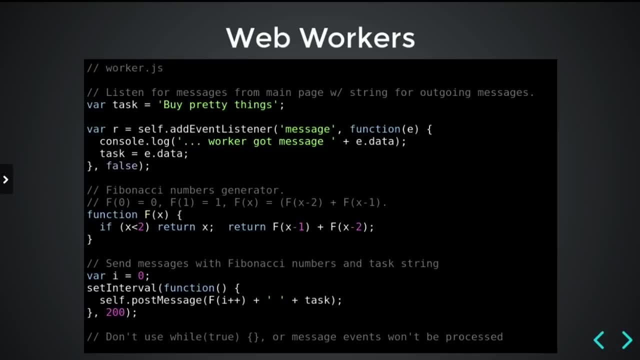 for these outgoing messages. So when we get into this, we find self right, And that's us. And now we're going to add this event list and this is just like we did on the previous page, right? And so now we're going to say: okay, worker, got a message. 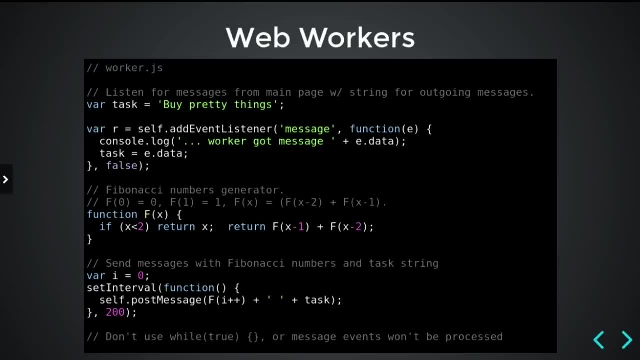 This is a horrible Fibonacci number generator. It's designed to be very poor performance, but it's designed like that to show the value of the web worker Right. And then here we are going to, so this loop here. this is where that wild tree didn't. 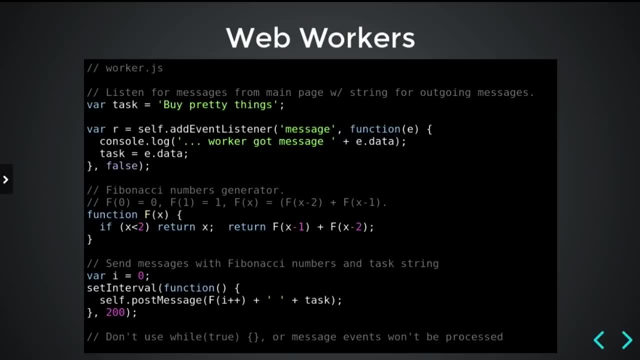 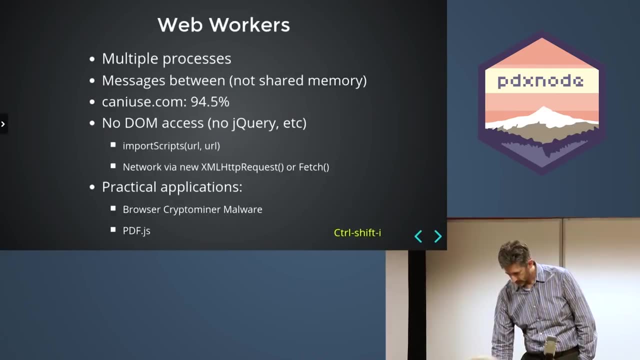 work. So here we set an interval and then, every 200 milliseconds, we calculate Fibonacci number and then we send it back to the index web page. So right, so this is a lot of the comments that we actually just talked about. questions. 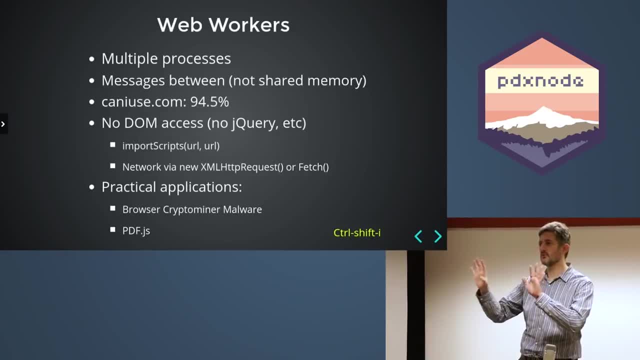 So, yes, you can do multiple processes right? We had those two scripts and now we had two event loops running so we could get two CPUs going. We can use this in about 94% of browsers. Like I said, no DOM access. 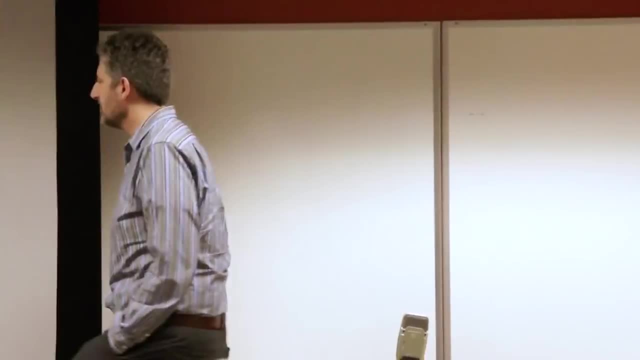 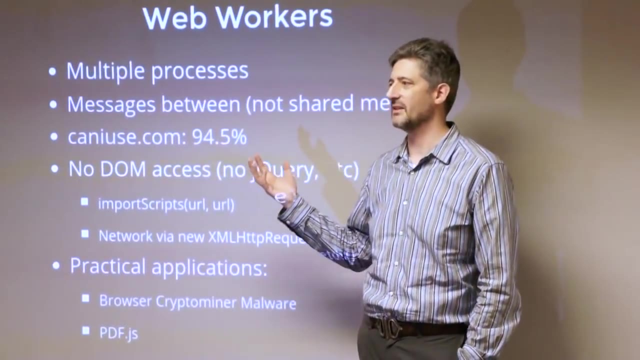 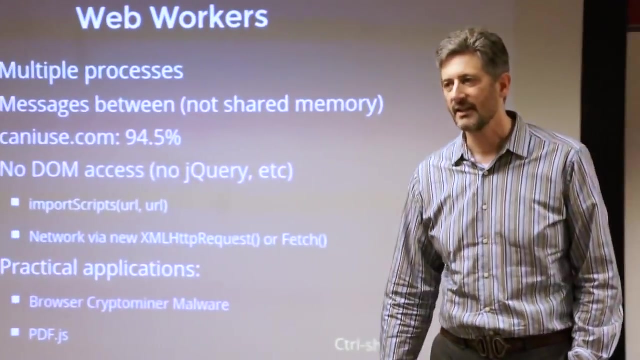 And in terms of practical applications. One of these is the CryptoMiner malware. Like that makes a great web worker right, Because you can just spin up all these CPUs that are not being used for any reason. And then another one- my sister pointed this one out to me- which is PDFJS, which is a 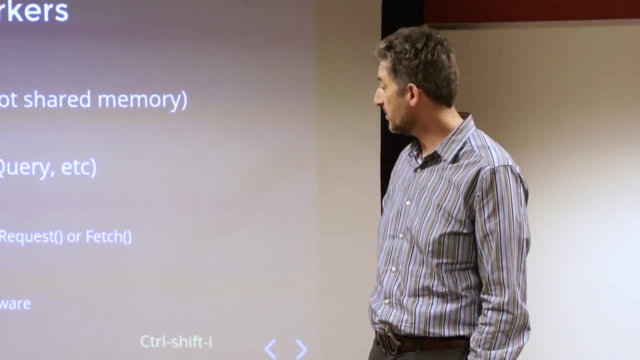 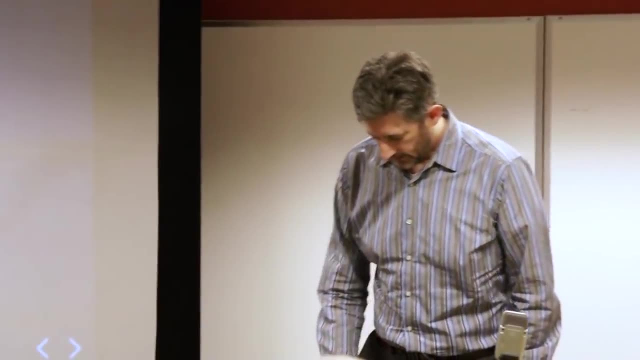 library that will process PDFs on the browser, And I think it does it through web workers. I was putting her on the cover and I thought that was a pretty cool application. All right, So you guys remember the code we just looked at. 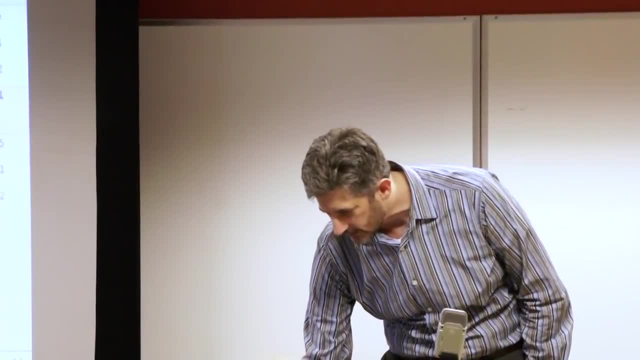 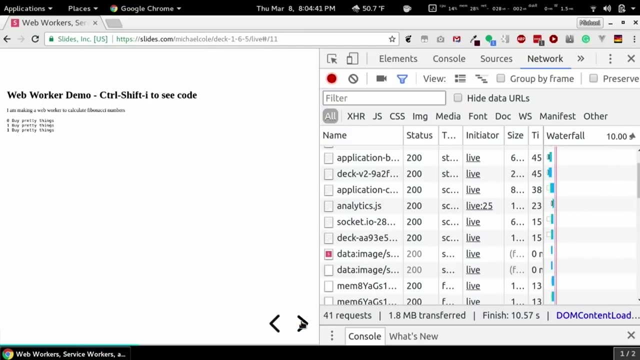 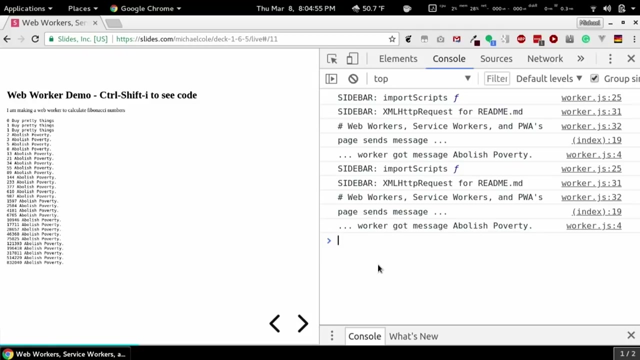 So here's that code in action. So we're going to go there And now we're going to look at this And sorry it's so small, but you can see that we're running, we're getting our Fibonacci numbers And now okay. so if you go to that GitHub, you'll see there's a couple. 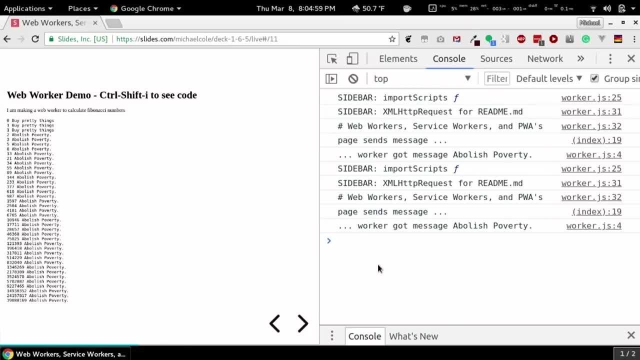 I added these like sidebars So we could do import scripts. We could also do So. here's our HTML request. So you've got to read the read me And this is text from the read me. Here you can see where the page actually sends the message. and the worker got the message. 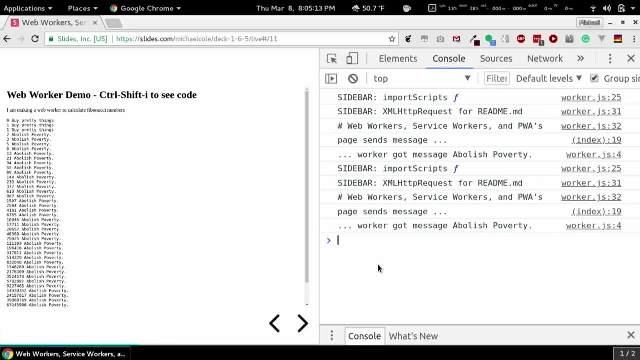 abolish poverty. Okay, We ran this twice And then, when we got that message, we changed from buy pretty things to abolish poverty. So that's it. So this is an example of our web worker. I think our web worker is still going down. 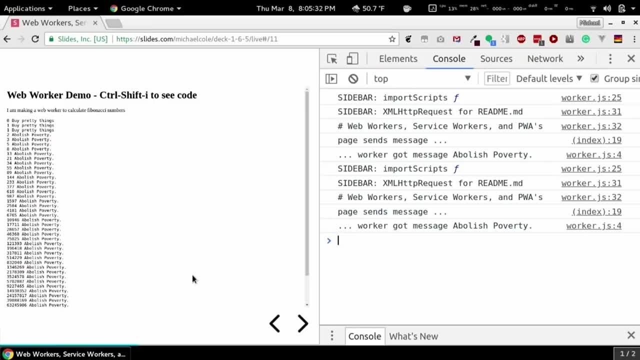 So if you guys can see my CPUs, you know. so we have 104 CPUs, So we're still, we're using like 100% of a CPU in this page, but it's still responsive And if we didn't have the web worker going, we'd probably get that unresponsive page. 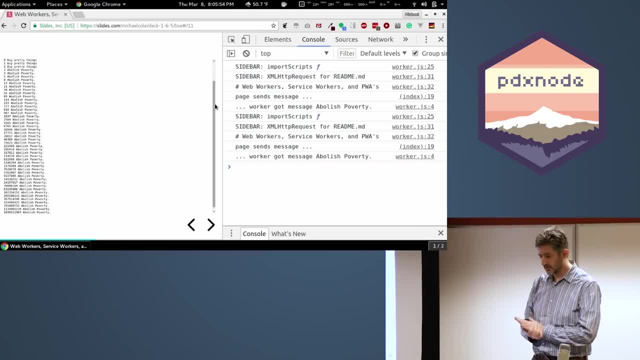 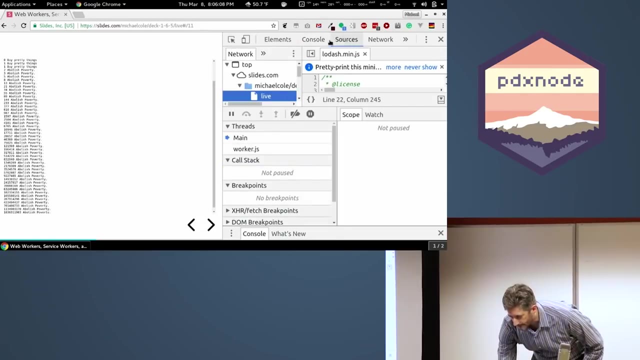 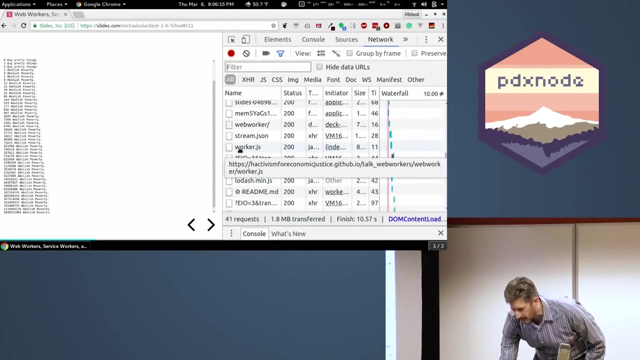 like Facebook page, right. So that's really the value of web workers. All right, Do you guys have any questions about that, about what happened here? Yeah, Yeah, Yeah, Let's see here. Now, this is so. I'm a little. I'm a little improv, improv here. 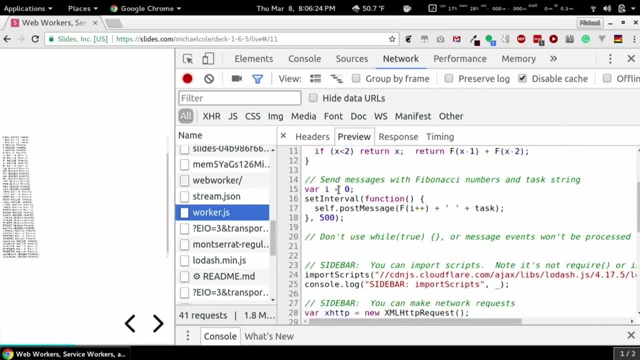 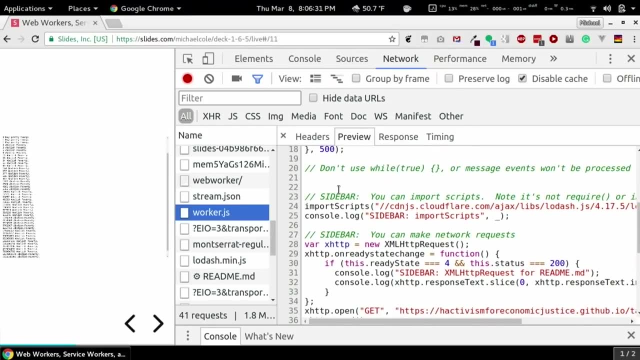 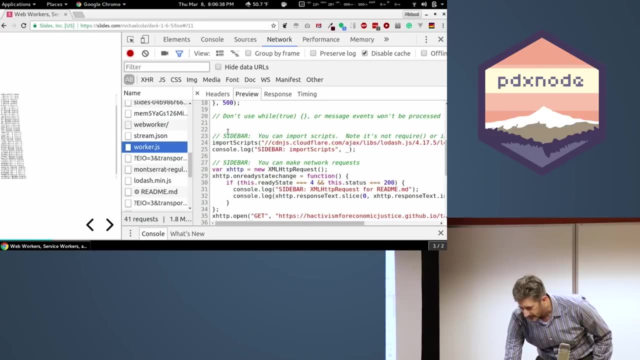 But I think we got it. Yeah, Yeah, And you know I'm a little bit jamming. It's like I'm the worst Fibonacci thing ever. So, like you said, right, Yeah, I don't know. 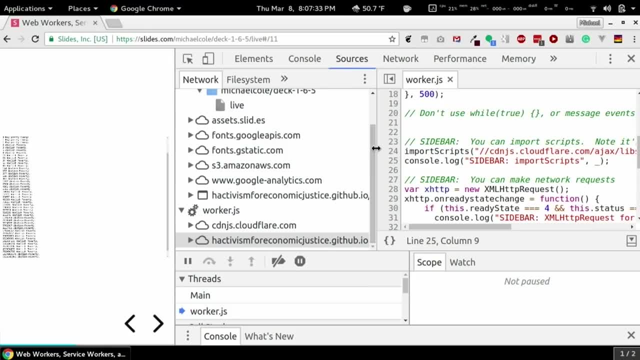 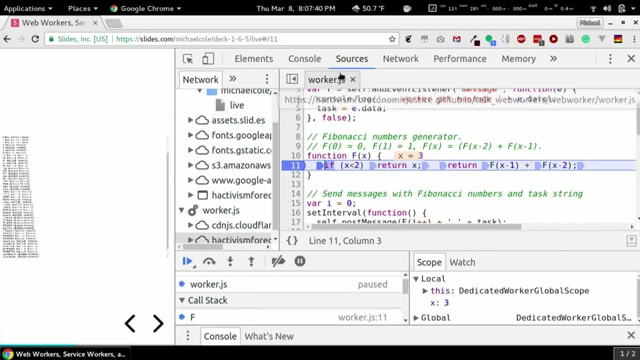 I wonder if that will happen. Let me try. let's try that. That sounds fun. Okay, All right, Right. And so it did break point, because you can see my CPU went down. All right, All right. 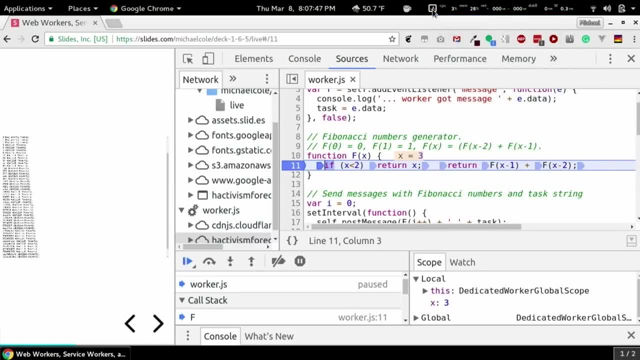 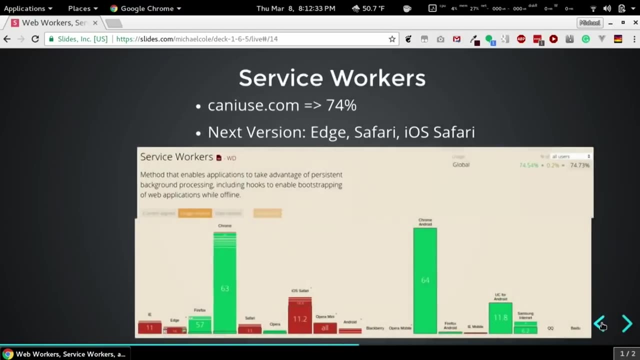 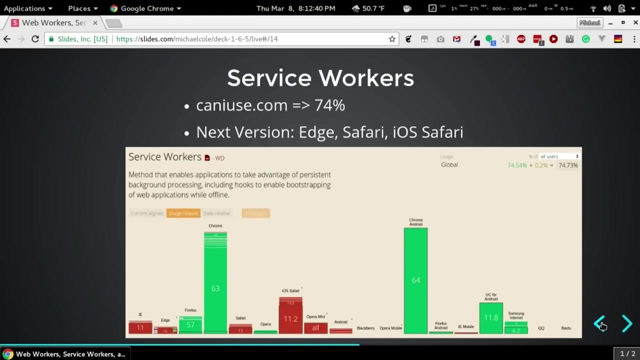 All right, can see my CPU went down. X is 3. yeah, nice service workers. now service workers are web workers. service workers have a can I use of about 74% and that's going to change in the next version of edge Safari and iOS Safari, so it's going to. 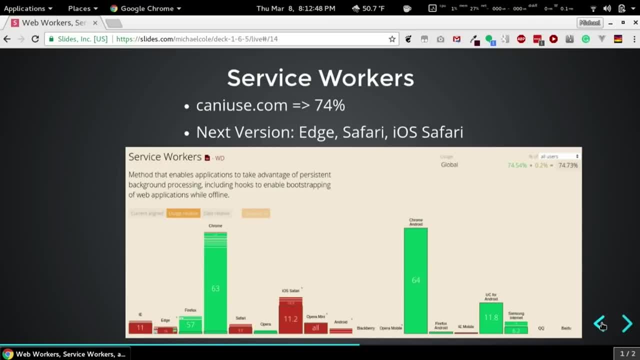 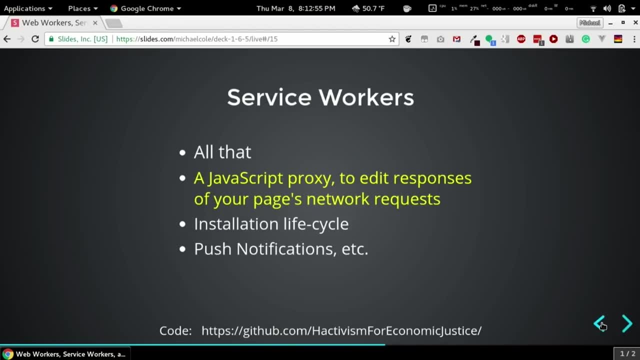 jump up to be pretty, pretty mainstream service workers, give you, like, all that web worker stuff. plus, you get a JavaScript prod proxy to edit responses of your page network requests- so we're going to talk about that- and you get an installation lifecycle, so it's almost like an app, and you get push notifications and other other app like. 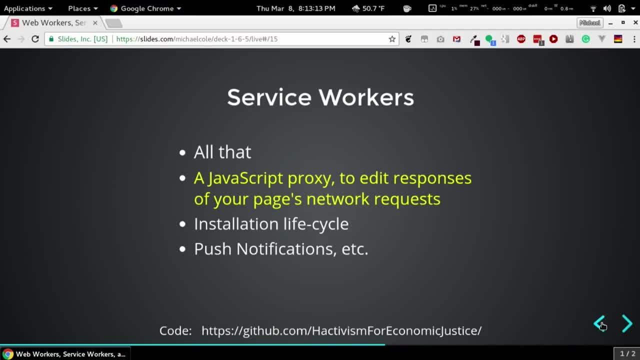 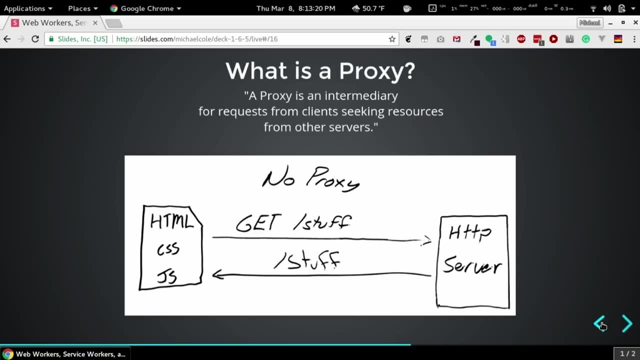 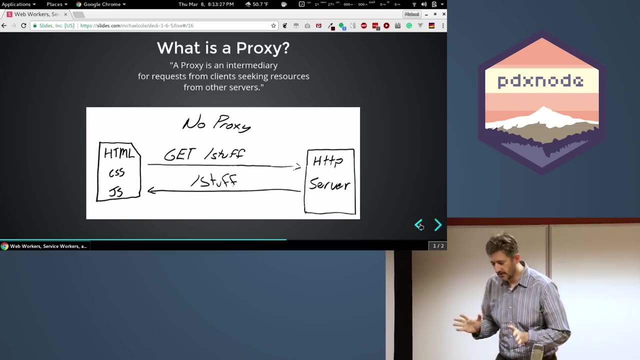 stuff. Google is really excited about PWAs. Google's really really excited about this. so how many of all y'all know what a proxy is? I don't like we should skip, okay. okay. so what is a proxy? a proxy is basically an intermediary for requests from clients seeking resources to other servers, so when my laptop wants to go, 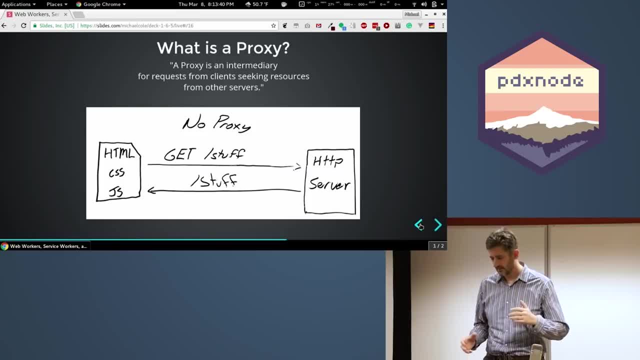 out and talk to slides, comm to get this presentation. it's on the, it's on the Wi-Fi, so the first proxy that it hits is the Wi-Fi. right, then that Wi-Fi access point is going to hit the upstream router, and that's another proxy, and so it's just proxies all the way up. it's. 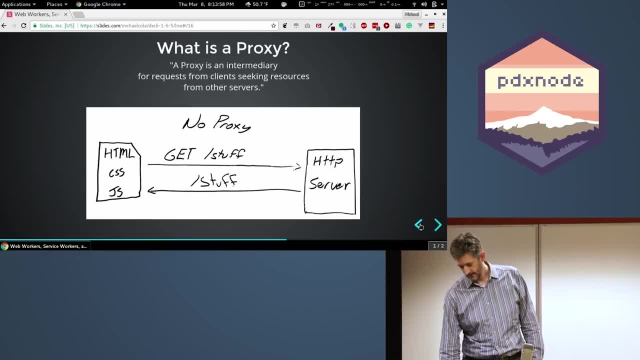 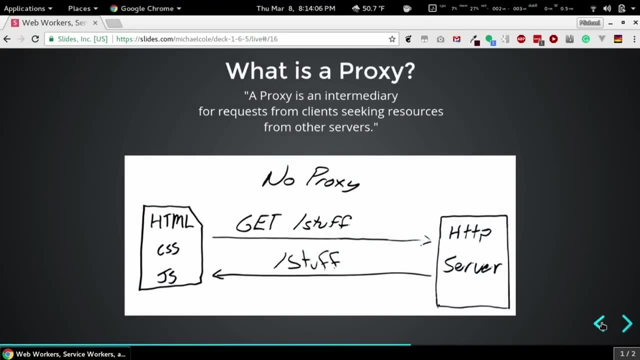 like turtles all the way down, proxies all the way up, and so this, so this, like this is almost like this, is like something that never happens, right? when is the last time you plug directly into a web server except on your light, on your? you're developing on your own computer, right? if you're using the? 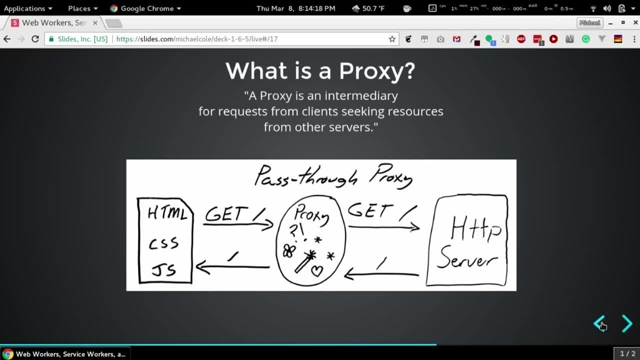 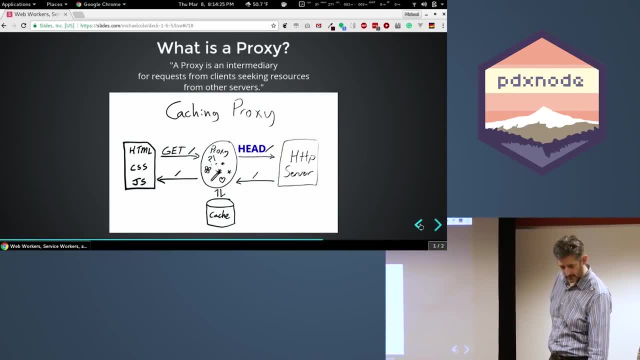 internet. you're getting a proxy in the middle and you know they could do all kinds of stuff. there's all kinds of stuff going on there, that et cetera, et cetera. yeah right, it's great, it's good. curse words: hearts, anti-blondes or marijuana cigarettes. 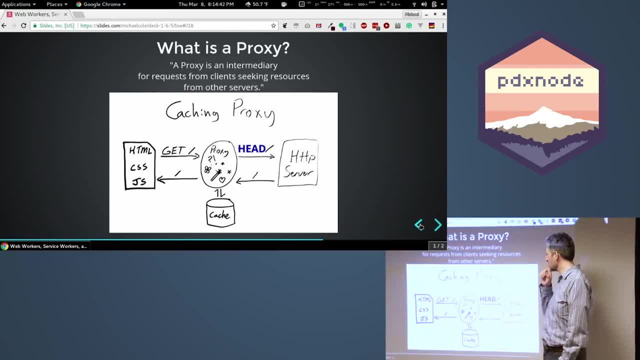 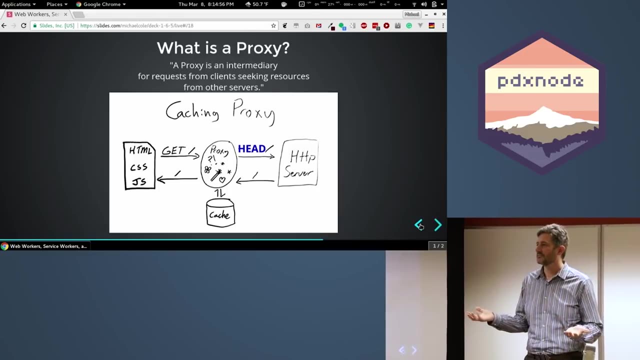 it could be shhh. so we can also get a caching proxy. and if you've ever like you know, if you've ever, are you guys familiar with a caching proxy right? so, like a like a CDN, like CloudFront, is a caching proxy right. like I've got my, my website in a bucket, an. 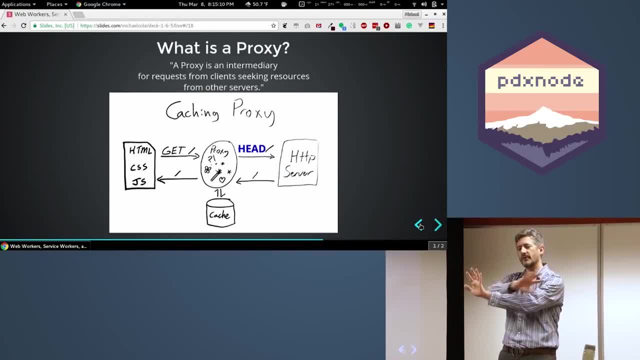 s3 bucket and then I put CloudFront in front of it and then, when the clients want the data, CloudFront only gets it when it knows it's out of date, right, so that's a really good. that's a caching proxy, okay. so if you wanted to do an, 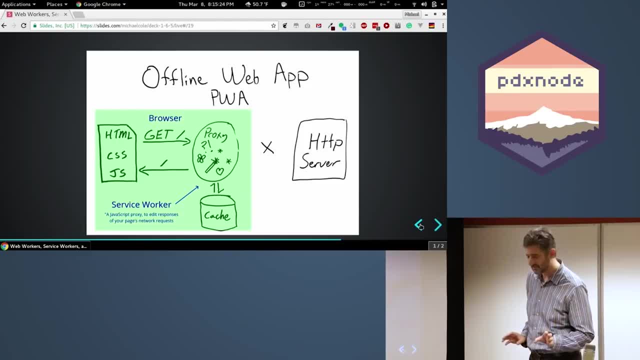 offline web app with a service worker. you could make something called a PWA. so then your service worker becomes the proxy, right, it has a proxy, a JavaScript proxy, to edit responses to your pages network request. this all happens in the browser and it has if you have a caching. and so then, if you don't have access to 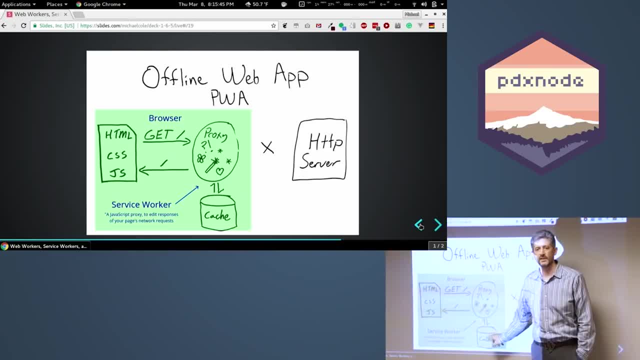 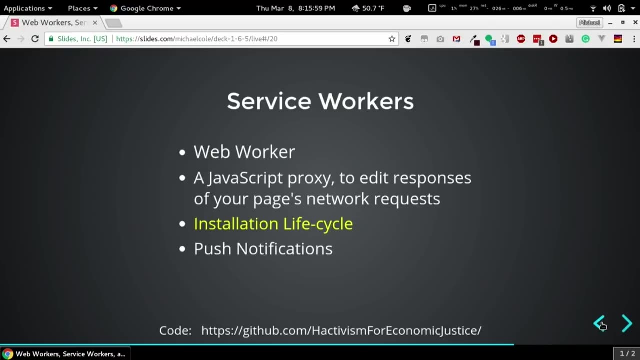 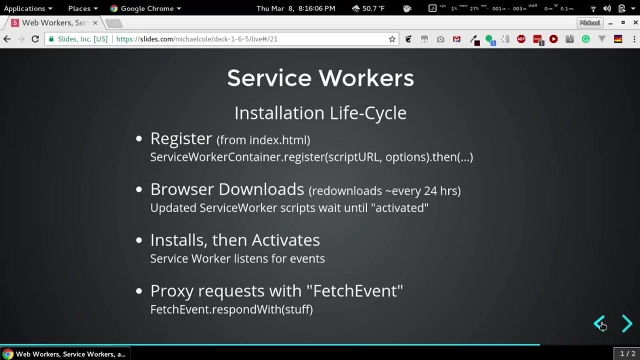 the internet, you can still make network work request based on the cache data. that's my attempt to explain that. how'd I do? all right, cool, all right. yes, thumbs up, I win. service workers also have an installation lifecycle, and so I'm gonna go over this just briefly to make you. 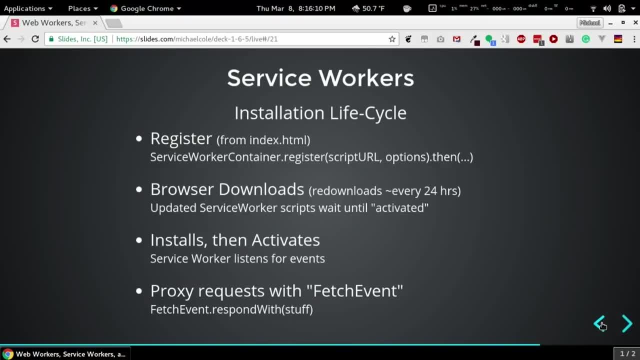 aware of it because it's kind of weird. it's like a new thing for web pages and there's tons of, there's tons of documentation. Google's really hot for this. basically, you can register your service worker like this, so just give you your options and promised, and then the browser will will download your service. 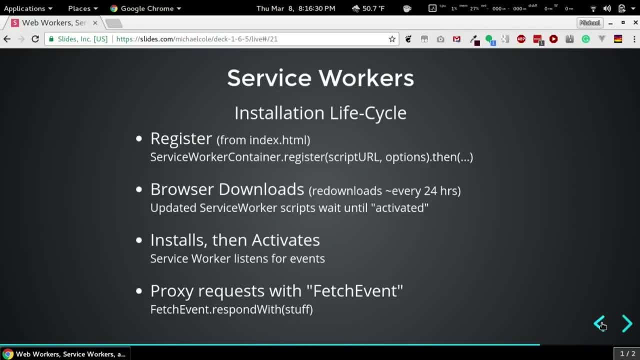 worker about every 24 hours and these scripts will, if they're updated, they'll wait to become activated. so we'll see this. we'll see this gonna happen a little bit. but then the service worker really just listens for events and then whenever there's a fetch event- so network requests- we'll go through a. 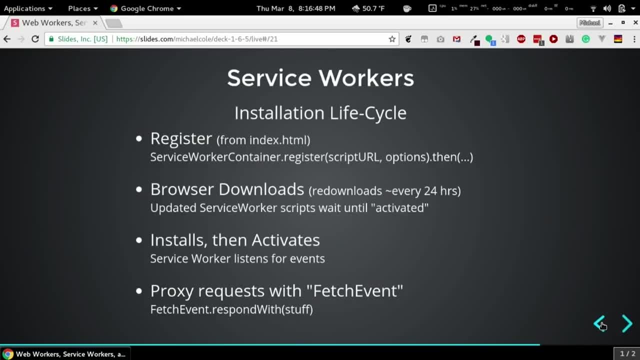 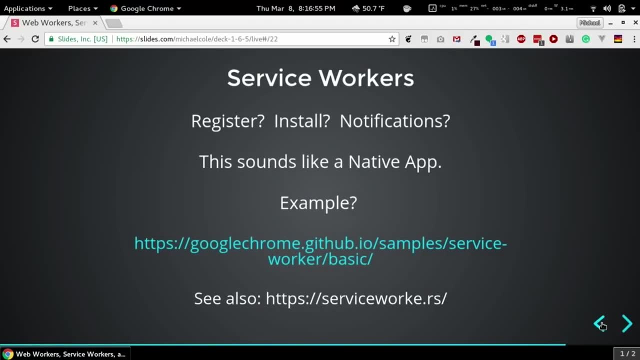 little fetching event and we can respond to stuff. all right, this is like I already- I think I already jabbered on this, but yeah, it's really kind of like a native app. it's kind of cool, in fact, I think. I think Chrome and Android are going to. 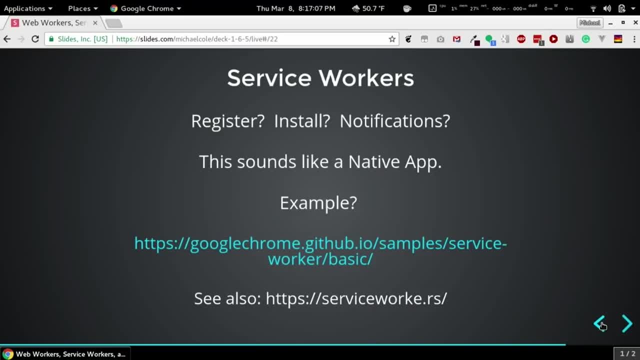 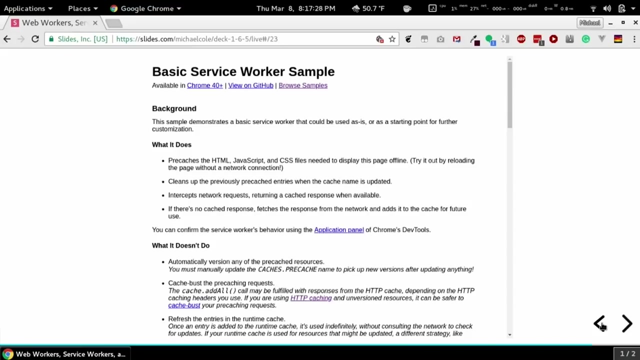 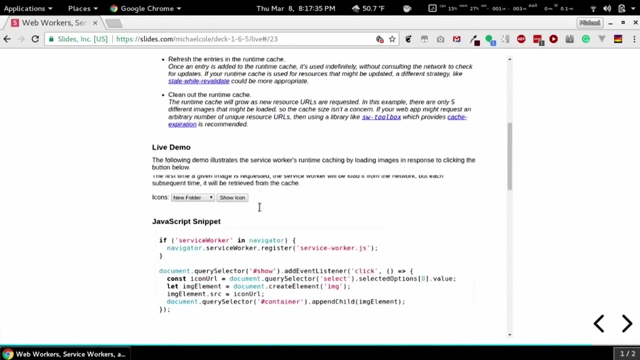 make API events to put it on your phones like desktop right, so you can get an icon with it. this service, workers, has some really good examples on it. if you want to see some really cool examples, I'll show this basic one and let's get into this. all right, okay, so so this bit here is the demo, all right, and it's. 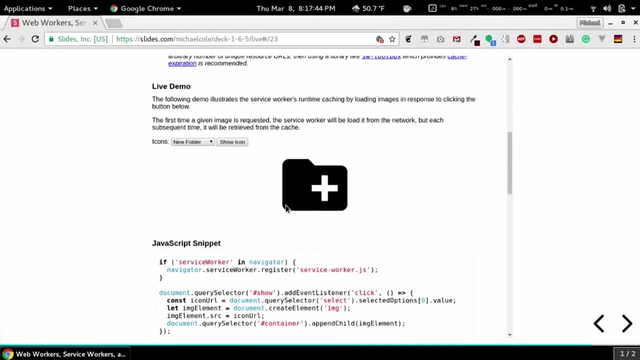 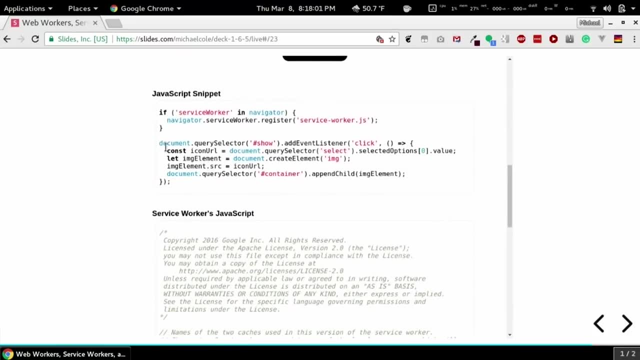 it's really just this one, we're gonna show icon. so really we're just gonna look at kind of the code that's going on in this, this bit here. so so here's where we, here's where we register our service worker, right, and then this bit of code: 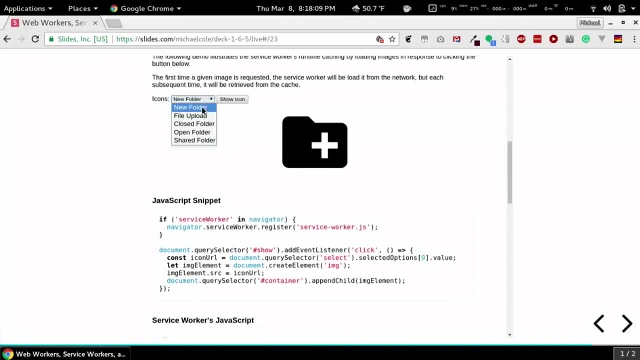 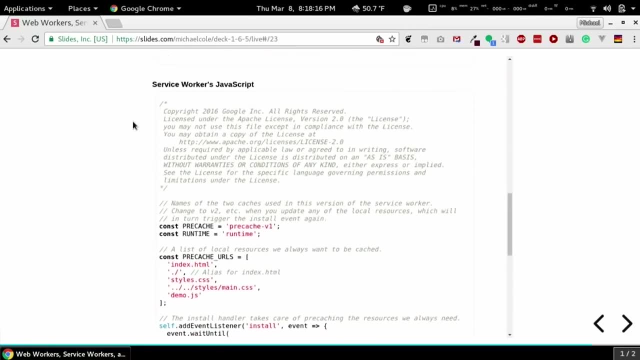 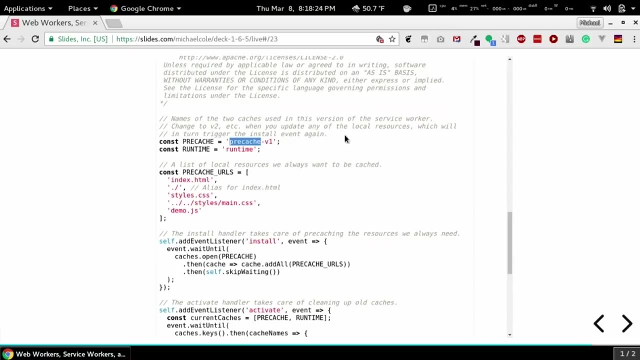 is basically the UI code for what's going on here now in the service worker. we're gonna- we're gonna have these named caps is and you can, you can update the caches as you go. so these are a pre cache URL so we can pre cache basically resources that we need for our application. you. 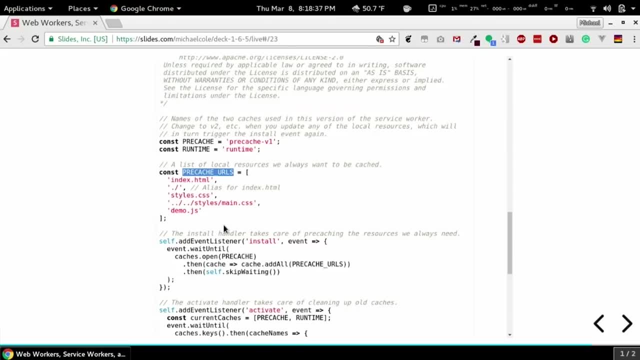 guys remember app cache, or was it application cache? yeah, like I think I think it's most famous blog post was application cats sucks, or something like that. so so this, this is kind of like this was. somebody was like, alright, let's do something better, so we came up with this, so here we can. we can basically pre. 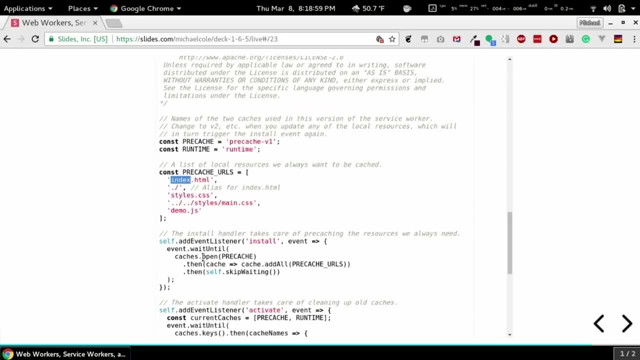 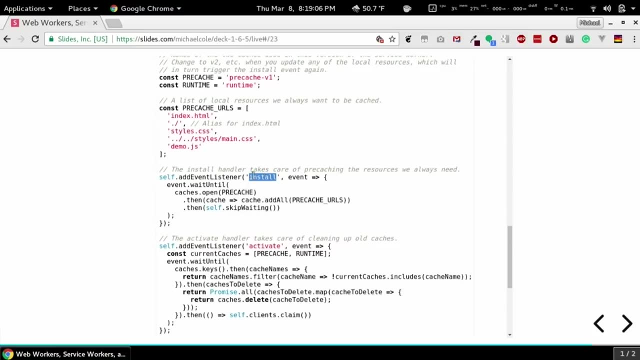 cache this index HTML and all of our stuff we need for the app. so then we listen for the install event and and when install happens we basically wait, and then we're going to go to our caches and we're going to open this pre cache cache and then we're going to cache a bunch of 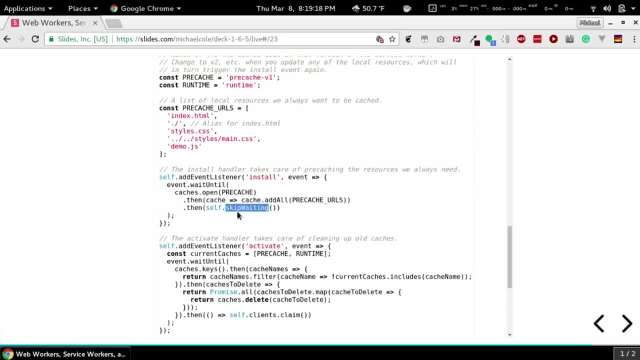 stuff. and then this skip waiting will activate any service workers that are waiting to be activated. do you guys remember that bit? all right, I hope you do. that's what it does the service workers if you. if you update the service worker, it'll wait until it's it's activated before it starts running all. 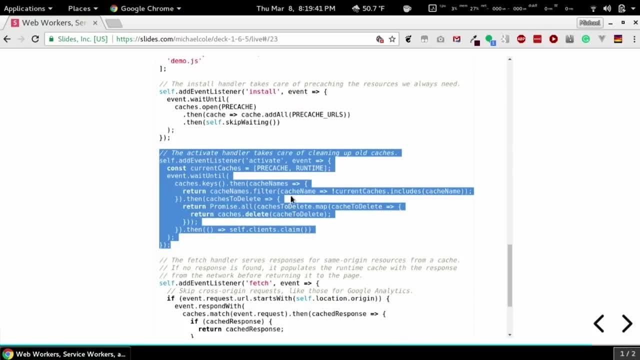 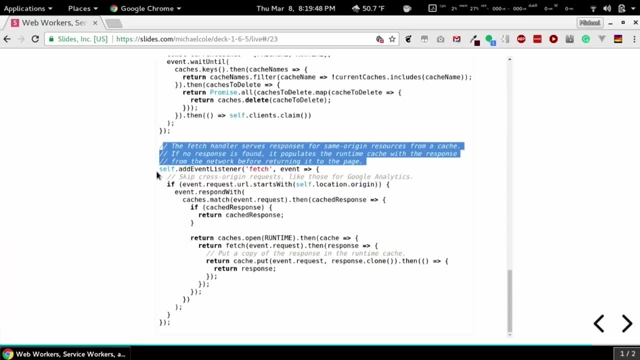 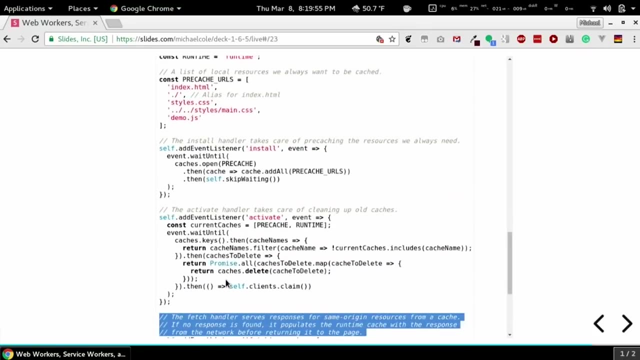 right. so then this bit of code here is really just cleaning up the old caches. if we, if we, made a new cache, it's not that awesome. but then here's the really interesting part where we talk about the proxy, right. so all of this, all this stuff is just a regular service worker. right, we were adding listeners and event. 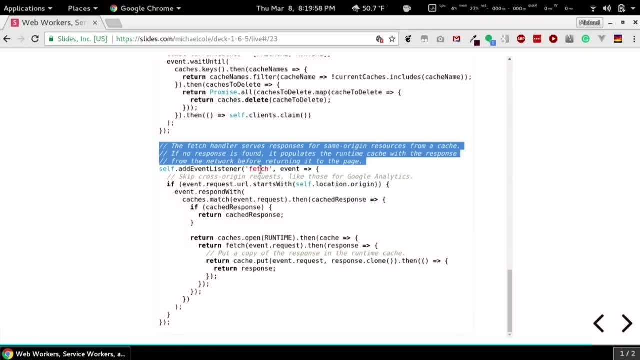 and all that kind of stuff. then we get down here and we get this fetch event. so this fetch event is when we get a network request, and I think this is a Google page, so you can see, here they're very concerned about Google Analytics, and so what we're saying is if, if the request starts with our, you are. 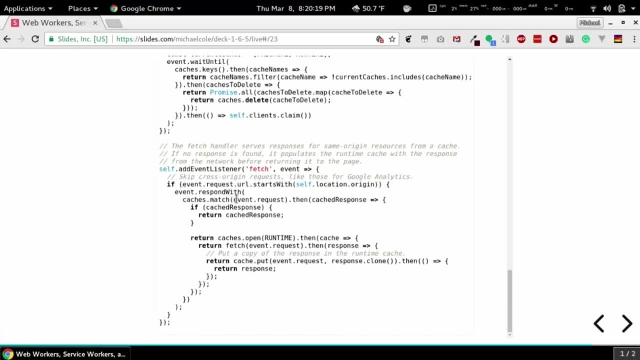 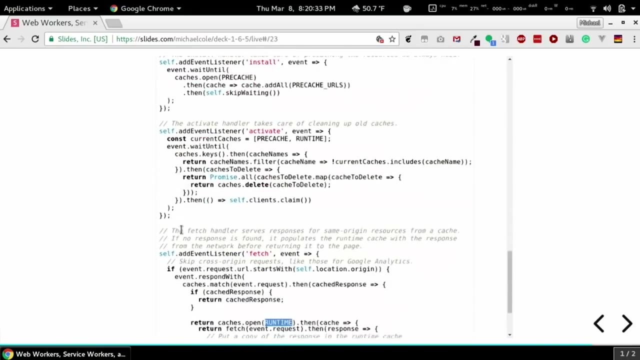 you our location, then we go to our caches and we try to find a match for the request and then we just send the response, right? so if cache response and response, if not, then we open the runtime cache- right, you remember the runtime cache? and then with that cache we run fetch to get the request and then we add: 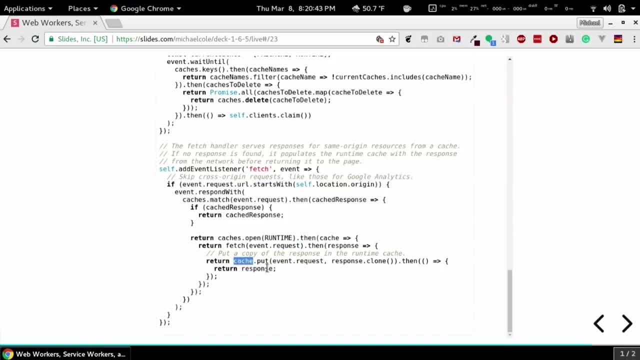 the response. we put the response into the cache and then we return the response right. so I mean, that's pretty, that's pretty much the gist of it and and with this, between the pre cache URLs and this bit, here we have everything we need to make an offline web app right. you can cache all your images, all your resources, all.